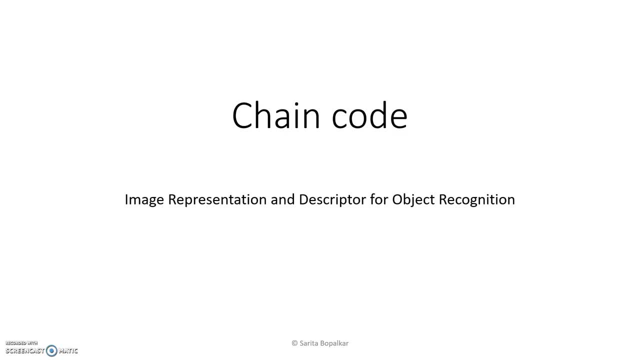 In real world, we humans perform this object recognition very easily and instantaneously. Like when we observe a scene, we can recognize tree, car and different objects. 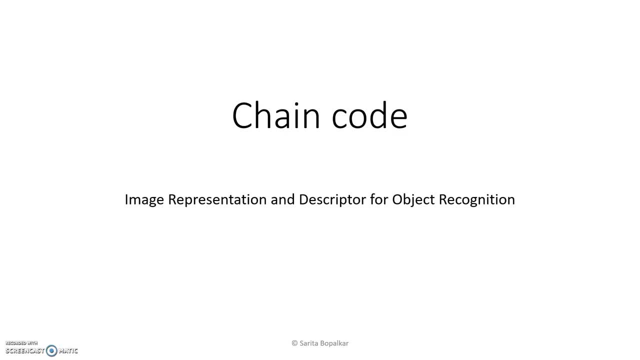 But to implement this object recognition on machine, we need to develop an algorithm. Let us see what are the steps in this object recognition. 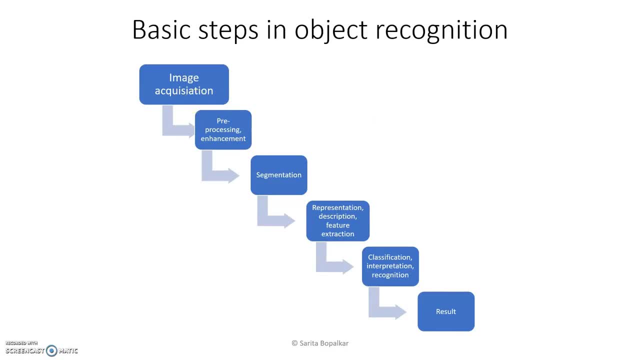 First step is image acquisition. When we get to the object, we can see the image. We can see the image, process it like enhancement technique, pre-processing to get a good quality of image. 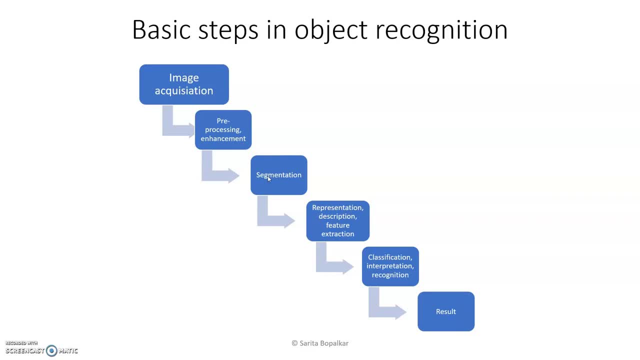 Then we segment the image into different segments. Some segments correspond to the image object and some segments correspond to the background object. After segmentation, generally we are performing morphological operations to regularize the image. 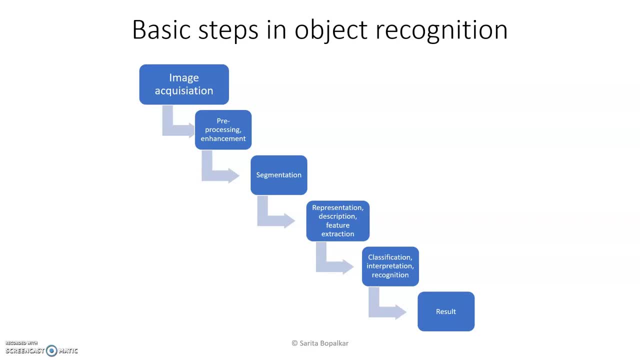 Regularize means sometimes different objects. Object may get connected by small line or on object there may be a noisy pixels. 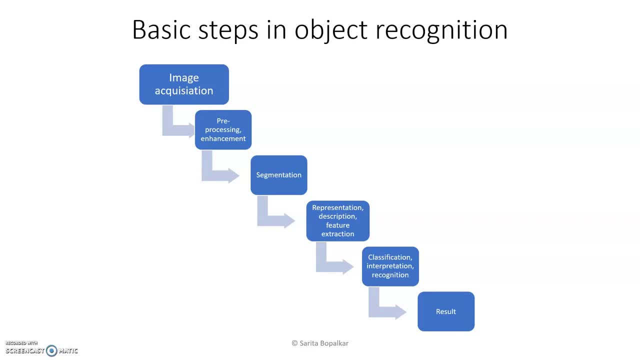 To remove that, we are performing morphological operations to regularize the image. And this fourth step is very important which we are discussing here. 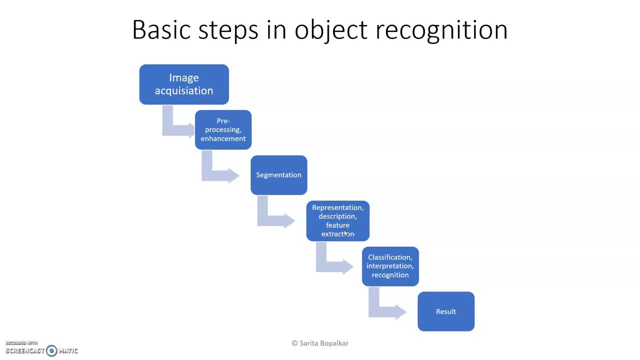 That is the representation and description and feature extraction. To recognize the object, we need to represent the object. 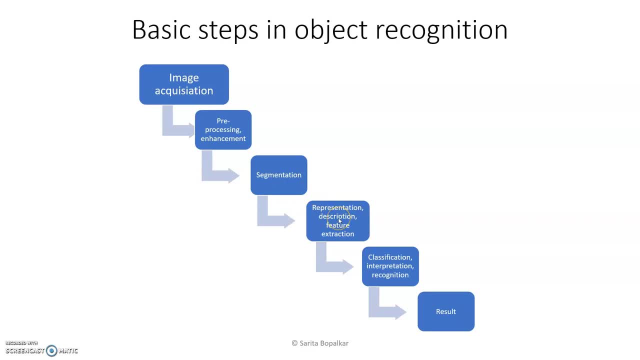 And from that representation, we need to obtain a descriptor. And this descriptor is compared to the descriptor stored into the data set of a machine or computer. 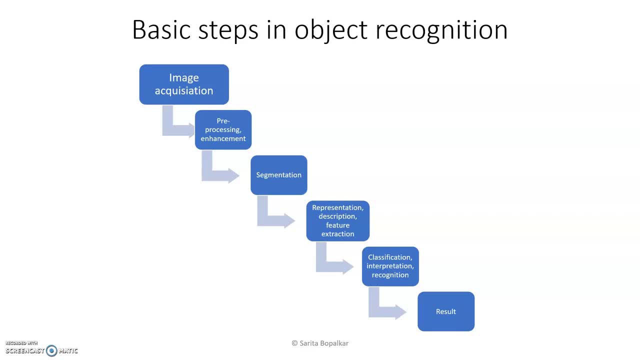 And when this match happens, we can recognize the object. 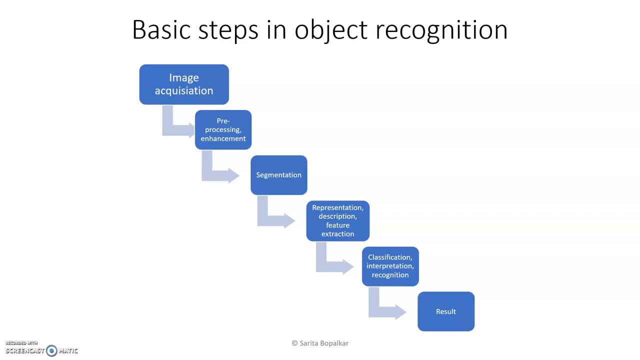 So these are the steps in object recognition. So here we are discussing this four point representation and description. 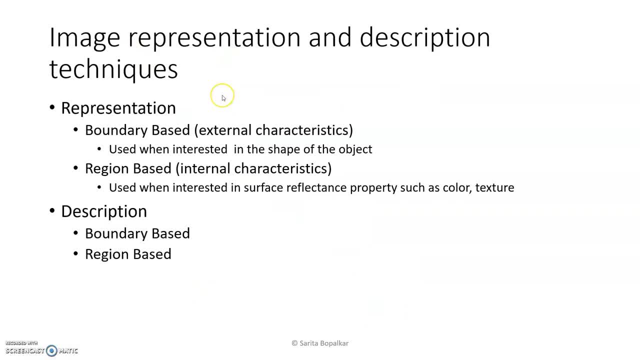 Image representation and description techniques are classified based on a boundary and region based. Boundary based representation is also called external characteristics. 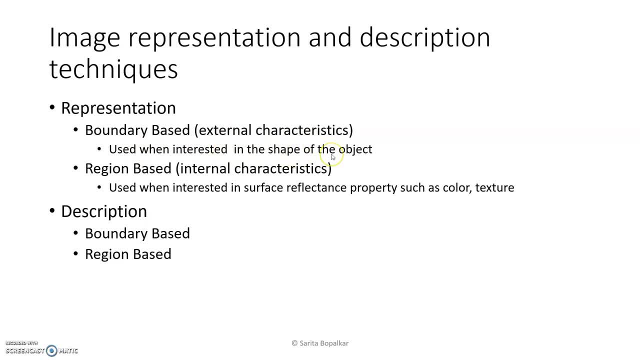 Means when we are interested into the shape of the object, we are going for the boundary based representation. And region based, we call it as an internal characteristic when we are interested into the surface reflectance properties such as, 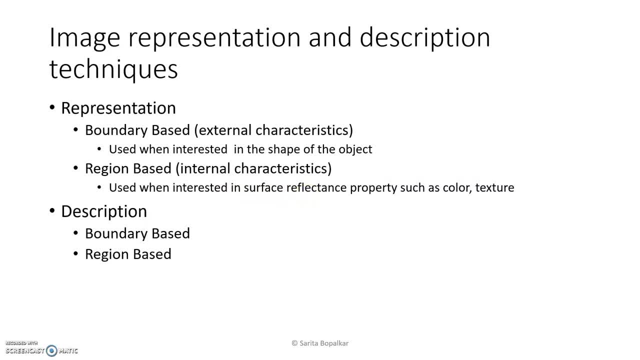 color, structure. Then we will go for the region based representation. 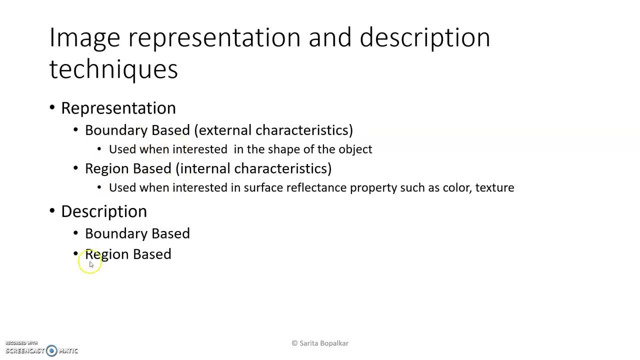 And from this boundary based representation, we can obtain boundary based descriptor. 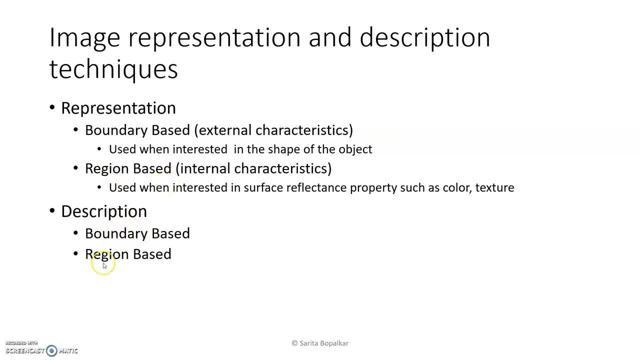 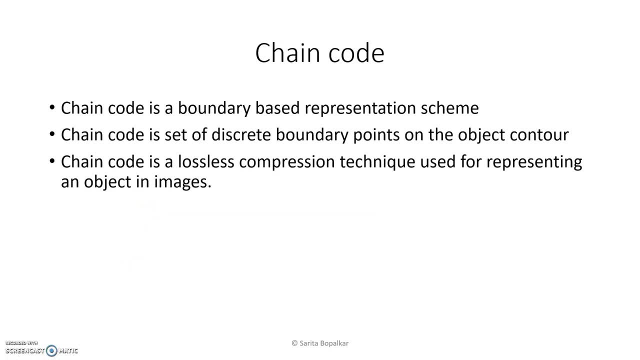 And from region based representation, we will obtain region based descriptor. Now we will start one of the boundary based representation scheme. That is a chain code. Chain code is the representation of the object. Chain code is a boundary based representation scheme. Chain code is a set of district boundary points on an object contour. Chain code, we can call it as a lossless compression technique used for representing an object in the image. So let us start how to obtain a chain code and why it is called as a lossless and how it is a set of district boundary points. Let us see. 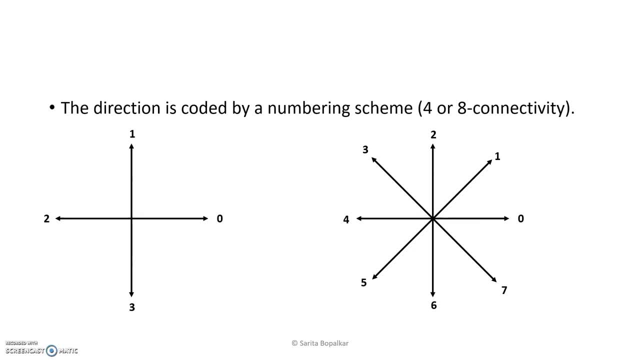 To obtain a chain code, we need a direction scheme. For that, we can use 4 connectivity or 8 connectivity. 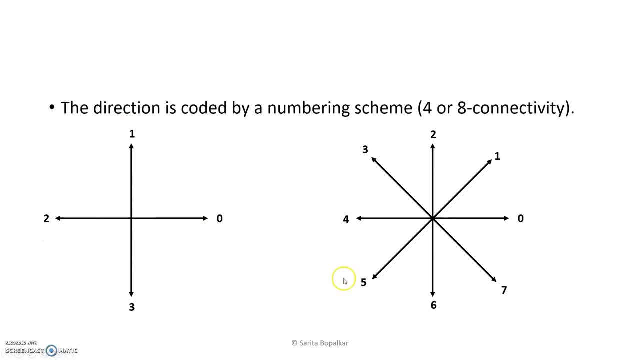 In 4 connectivity, 4 directions are there. In 8 connectivity, 8 directions are there. 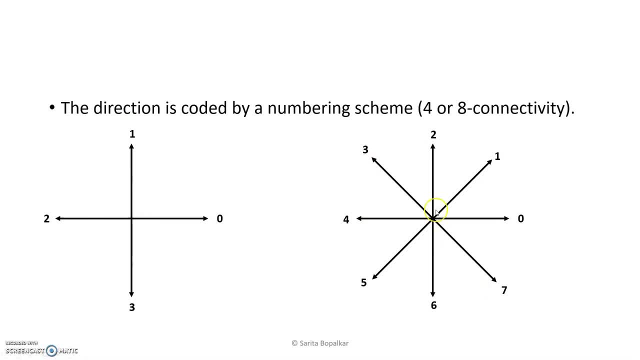 8 connectivity is very close to the human eye. Suppose this is our start point. Center point is our start point. Then to move to the next pixel. If the next pixel is in this direction, we will represent it as a 0. 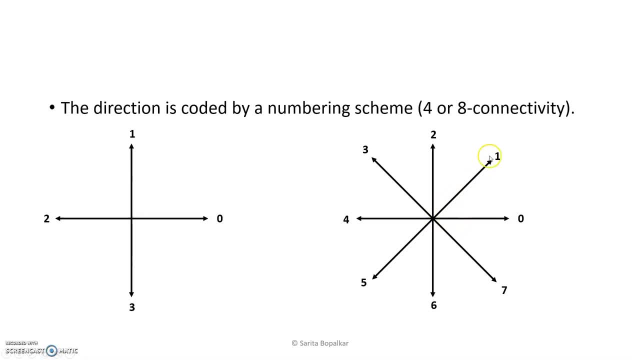 If next pixel is in this direction, we will represent it as a 1. If it is in this direction, it is represented as a 2. 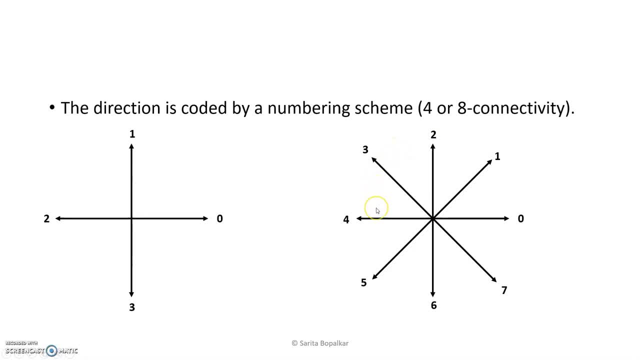 Like this, your direction code varies from 0 to 7. And in 4 connectivity, only 4 directions we are considering. 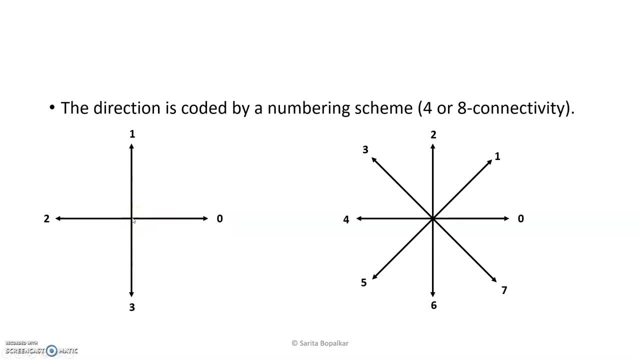 If this is your center pixel is your start point. If next pixel is in this direction, we will represent by 0. If it is in this direction. We will represent by 1. Like this, only 4 directions varies from 0 to 3. 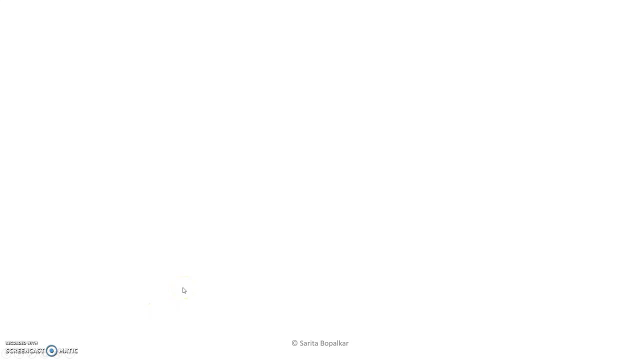 Let us start with the actual boundary points. Let this represent the district boundary points of an object. Now, to start the chain code. Let this is our starting point. To move from this point to this point. What is the direction convention? According to the 8 connectivity, we will assign one code. Then next. This point to this point. 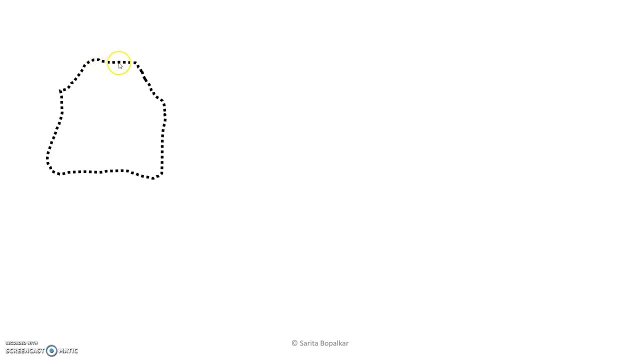 This point to this point. Like this, for each direction move. 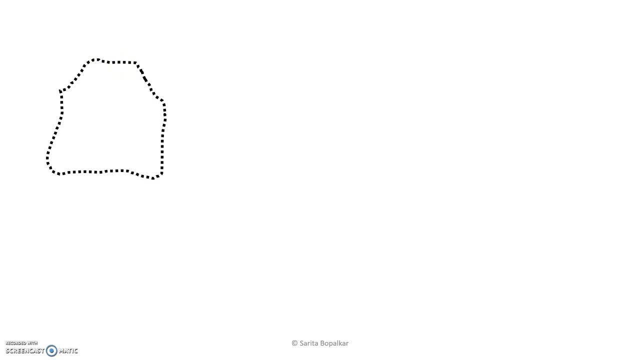 We will assign the number which varies from 0 to 7. According to the 8 connectivity. 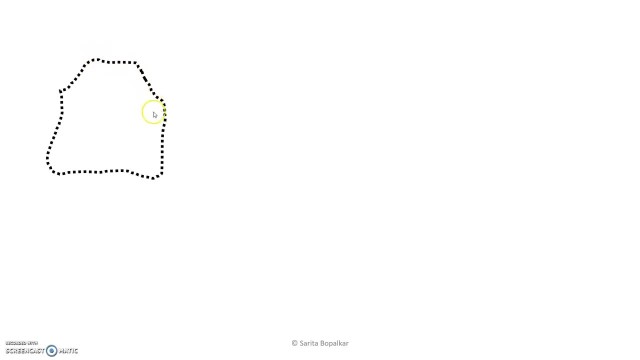 If we go from this direct district boundary points or original boundary of the district points. 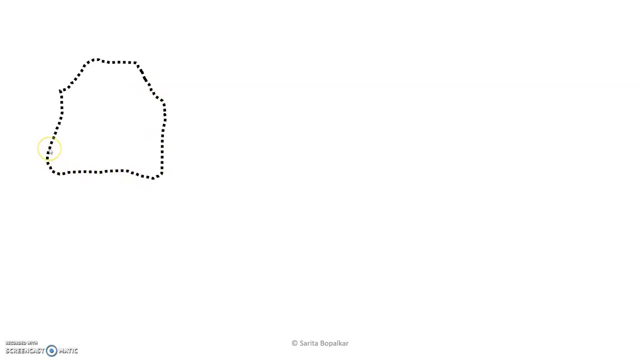 Your chain code will become too long. 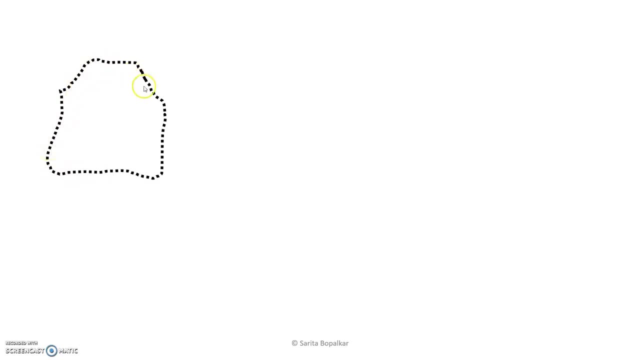 So, to avoid that, we are resampling this original boundary point. To reduce the length of the chain code. 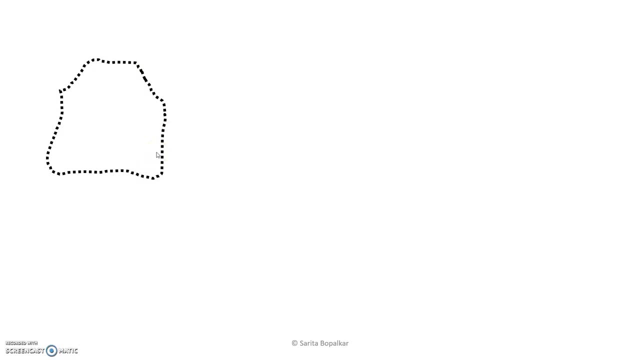 And how we are resampling? By assigning it to this grid scale. 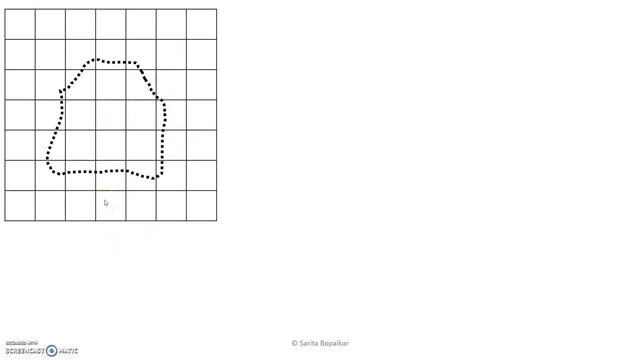 So, this grid scale is assigned to this boundary point. Now, we will assign a grid point to this boundary point. Which is nearest to the boundary point. So, this grid scale is near to the boundary point. Which will represent these boundary points. Like this. Next. This is the boundary point which represent these boundary points. So, we will select the grid point which is close to the boundary point. 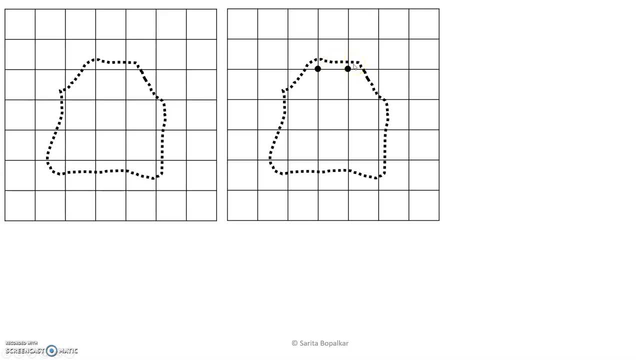 Or we can say which approximately represent the boundary points. 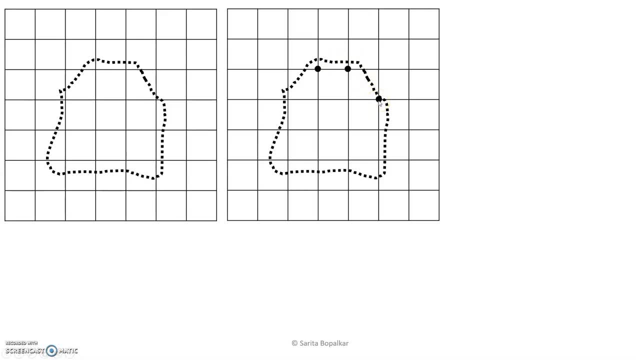 Next grid point will be this one. Next will be this one. Next should be here. Now, here. Next should be here. Like this. Next grid point should be here. Like this. 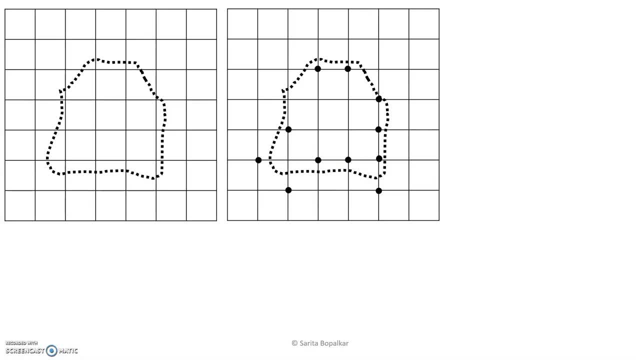 We will assign the different grid points to the district boundary points. Which approximately represent the district boundary of the object. 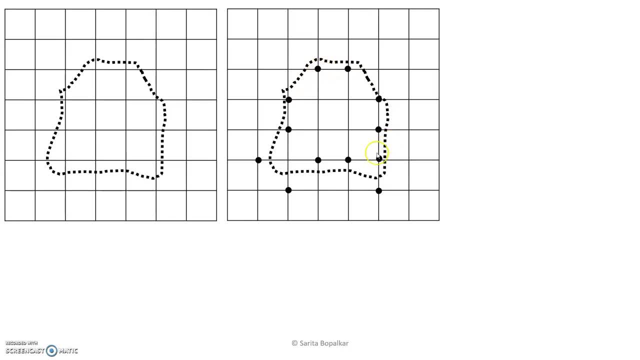 And we will generate a chain code for this grid point. Instead of generating the chain code for the district boundary. 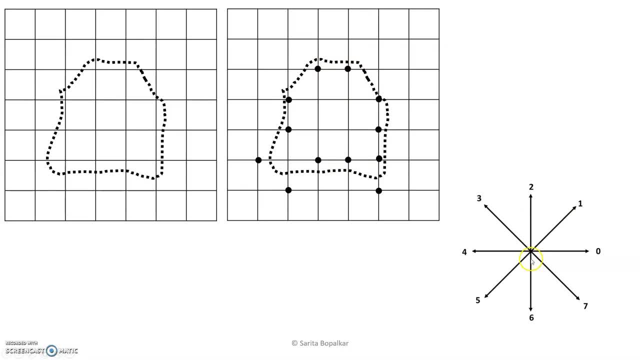 The sign convention here. We will use the 8 connectivity. Now, let us see how to generate the chain code for this grid points. 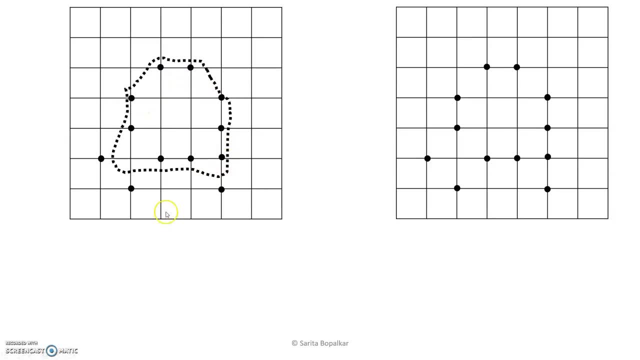 So, same grid points I have copied here. We need to decide the starting point. 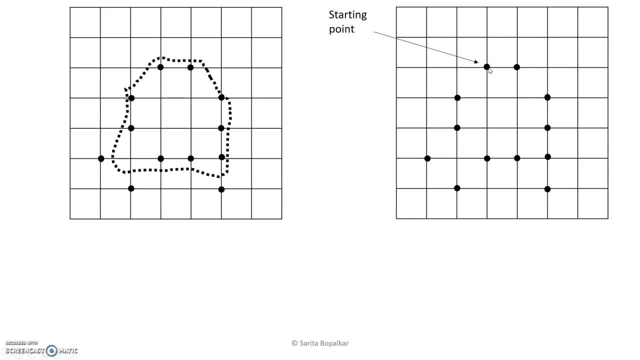 So, suppose this is our start point. Now, to move to the next grid point. This is the direction. Next grid point. This is the direction. Like this. We will decide. What is the direction required to move to the next grid point. So, these are the direction. 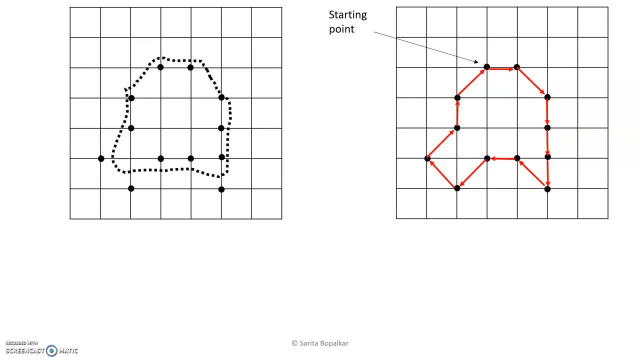 When we are moving from one grid point to the next grid point. From this starting point. 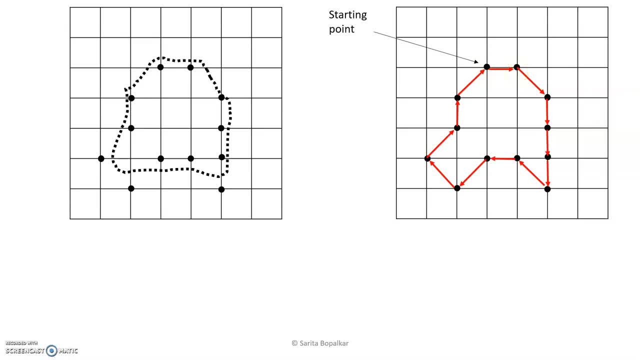 Now, we will represent this direction by a numerical value. For that, the direction convention is 8 connectivity we are using. 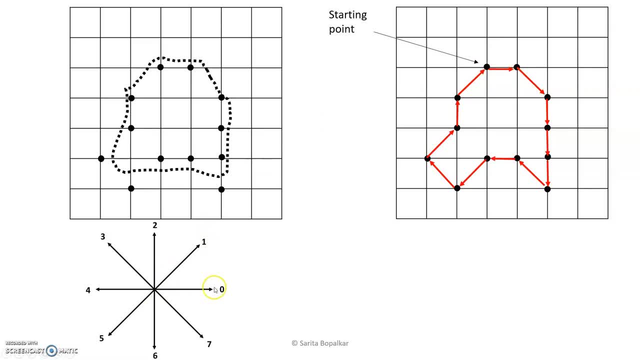 To represent this horizontal direction. The number represented is 0. 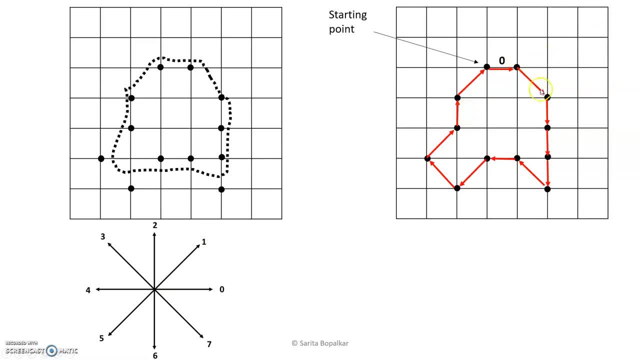 Now, this direction move from this point to this point. Direction is represented by 7. Like this. 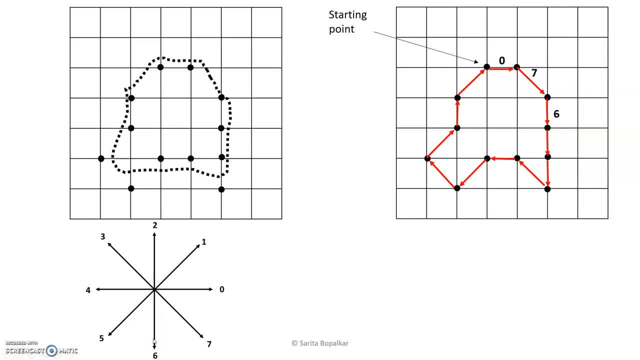 Next is vertically down represented by 6. Now, this diagonally upward into the left represented by 3. 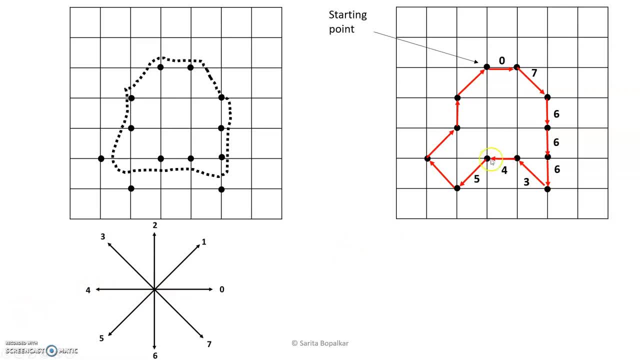 This direction is represented by 4. Here, this direction downward diagonal is represented by number 5. Upward diagonal is represented by. Upward diagonal in left side is represented by 3. Upward direction in right side is represented by 1. 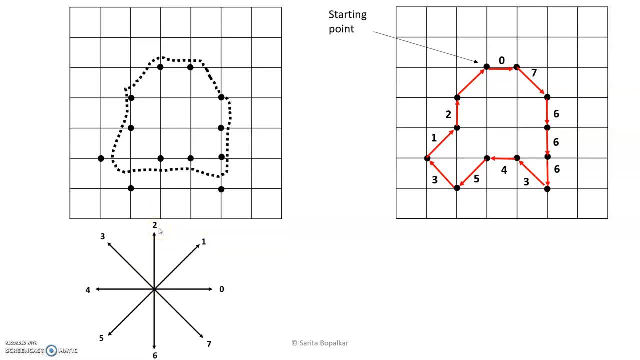 Vertically upward represented by 2. Like this. 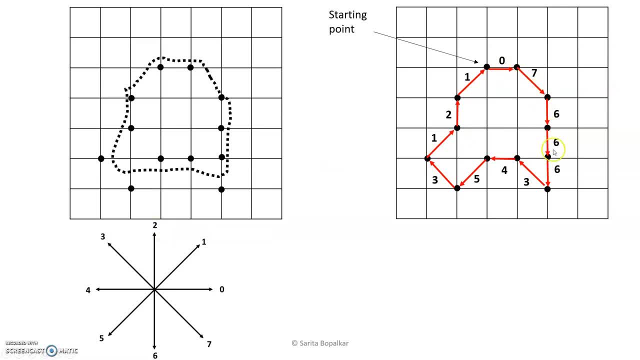 Each direction move we are representing by a string of a number. And your chain code is 0 7 6 6 6 3 4 5 3 1 2 1. 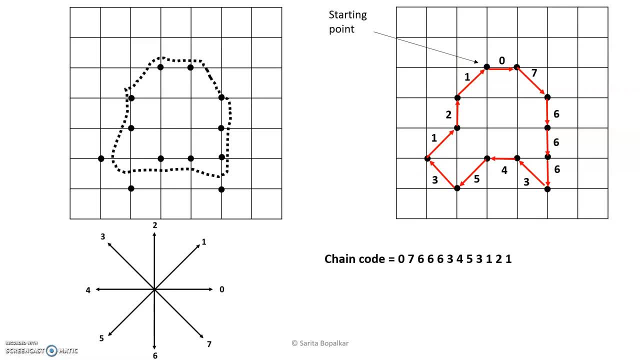 So, this is your chain code. So, what is a chain code? We are deciding a starting point on this grid point. And we will represent the move. Each move. With the numerical value. Now, we will try with the 4 connectivity also. 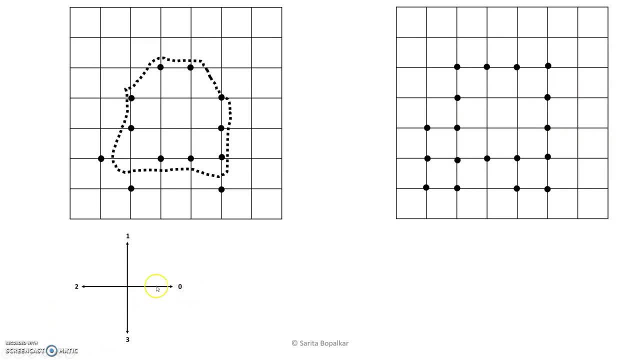 In 4 connectivity, there are only 4 directions. Horizontal and vertical. Left, right. So, we cannot consider the diagonal move. 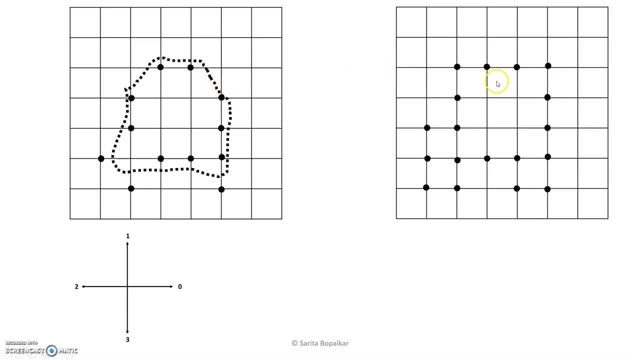 So, here we need to add the grid points. So, I have added a grid point where there is a diagonal move. 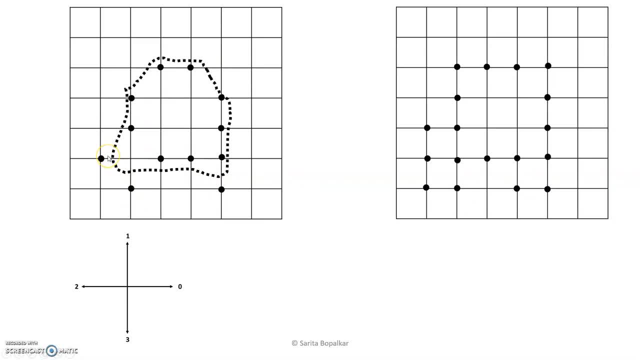 So, these are the grid points for the 4 connectivity. 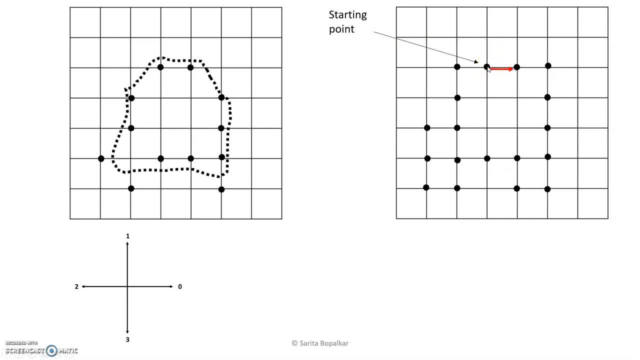 Let's decide the start point. So, let's decide the direction for each subsequent move. 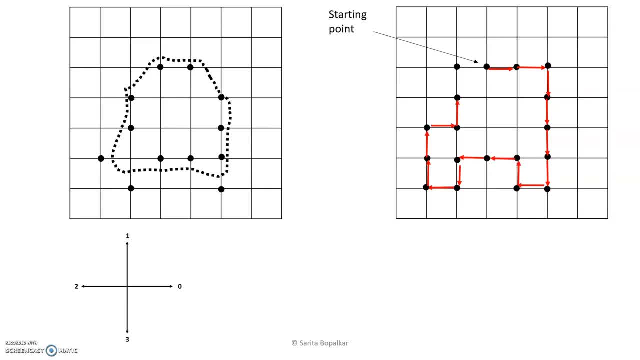 So, these are the directions. And we will assign the code for each move. 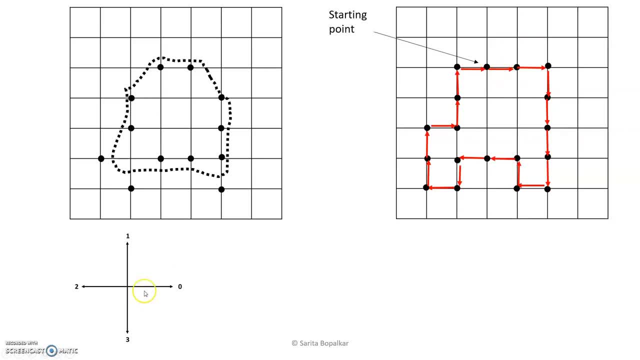 From the start point, this move is represented by 0. Next is also 0. Then downward is represented by 3. Again 3 3 3. Then towards the left, horizontal move by 2. Upward move by 1. Like this, 4 sign convention, 4 directional or 4 connectivity we are using to represent the direction move. 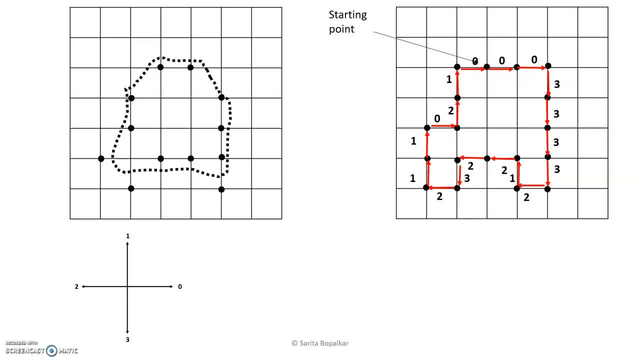 So, your chain code will become, yes, 0 0. Then there is 3 3 2 1 2 2 3 2 1 1 0 2 1. In 4 connectivity, we are considering only 4 directions. 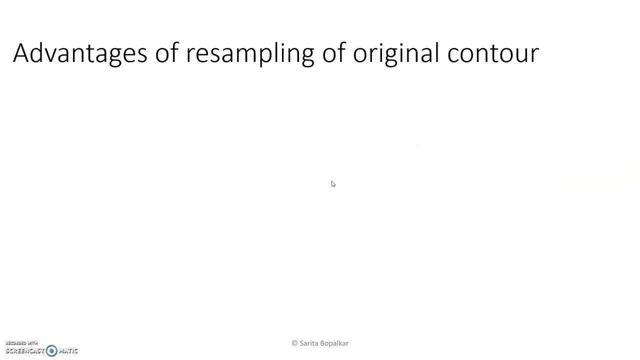 So, this is about the chain code. 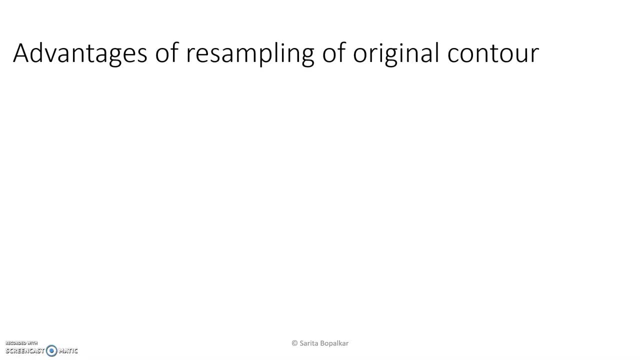 Now, advantage of resampling the original contour. What we did here, instead of considering the original distance, we resampled it. Let this is your original boundary point. If we assign the number for each subsequent move, you can check here, your chain code will become too long. 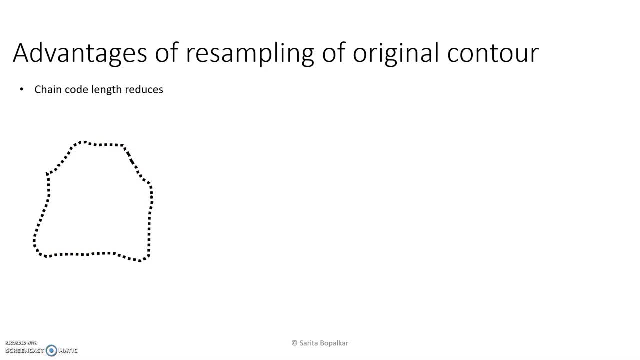 The resampling reduces the length of chain code. One more advantage is, we may get different chain code for original boundary due to discretization process or due to noise. Let me explain this. Let consider some subsequent points. When we are discretizing the boundary of the object, when we will get this district points, there may be error introduced into the discretization process or due to some noise, some point may placed at some another location. 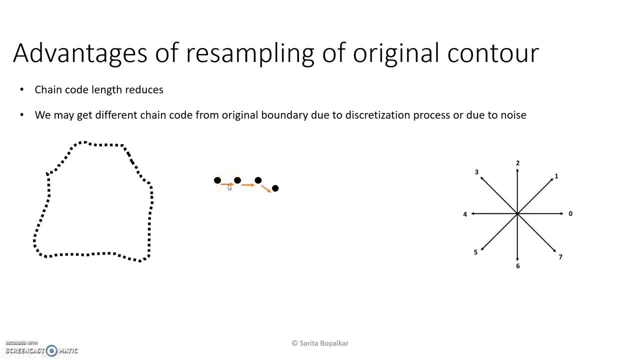 First, we will obtain the code for this one. According to 8 connectivity, what is the code? 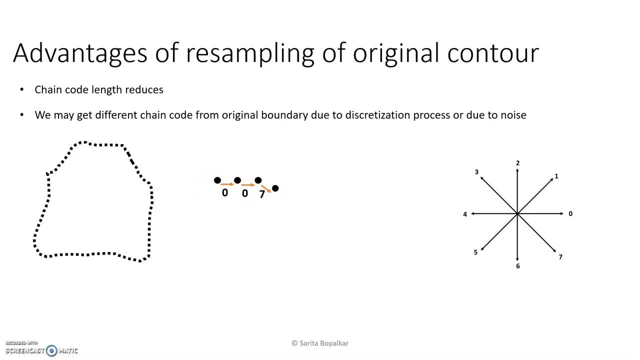 0 and 7. Now, due to error or noise, this point is slightly shifted upward. Now, what will become the chain code? 1, 7, 7. So, if you observe, the chain code is totally different from the original chain code. 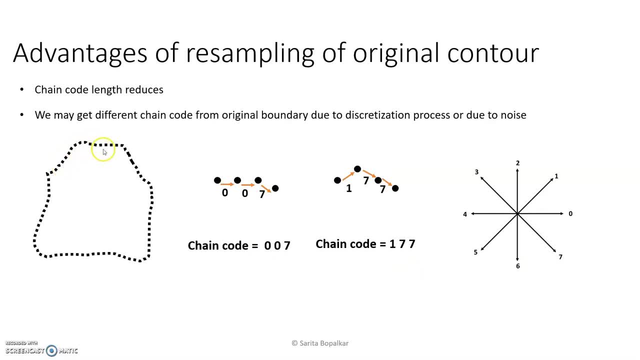 So, if we obtain a chain code from original district point, due to noise, you may get a wrong chain code. 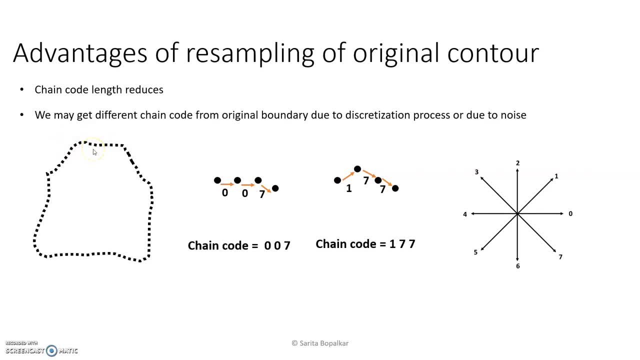 And if we resample it, this noise get reduced. 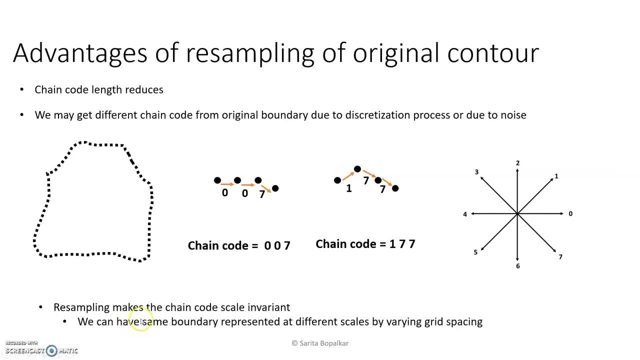 One more advantage of this resampling is, resampling makes the chain code scale invariant. We can have a same boundary represented at a different scale by varying the grid spacing.